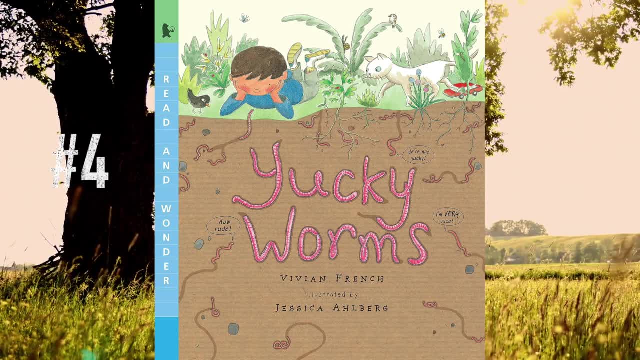 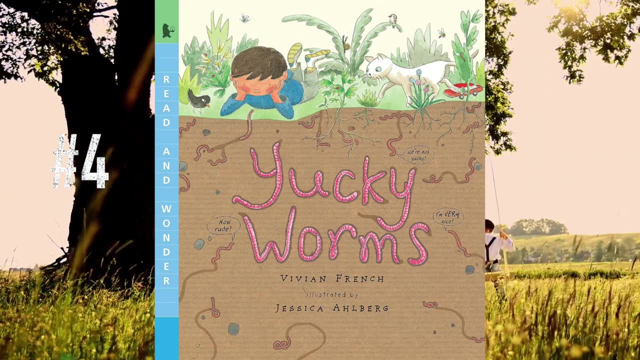 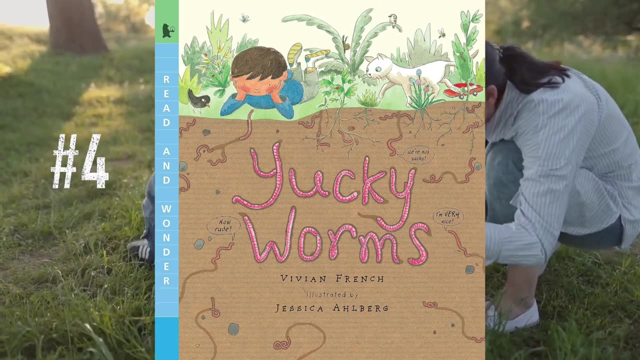 and why it's vital to life on earth. Number four is Yucky Worms: Read and Wonder. This book delightfully reveals why worms are wonders not to be overlooked. The author invites kids to appreciate the positive impact worms have through charming storytelling from a worm's wriggly. 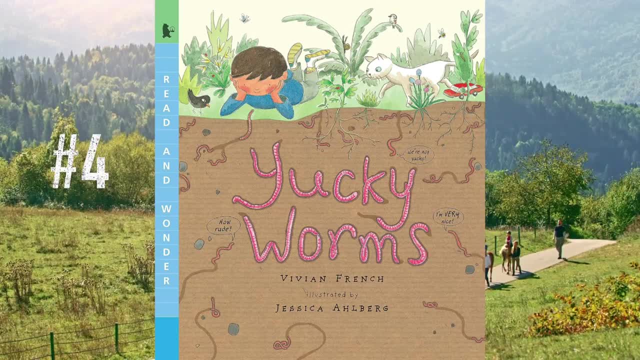 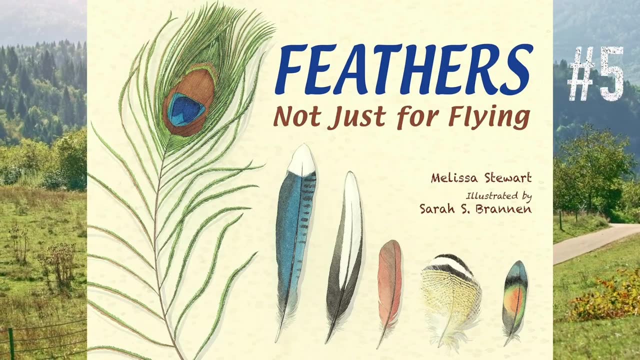 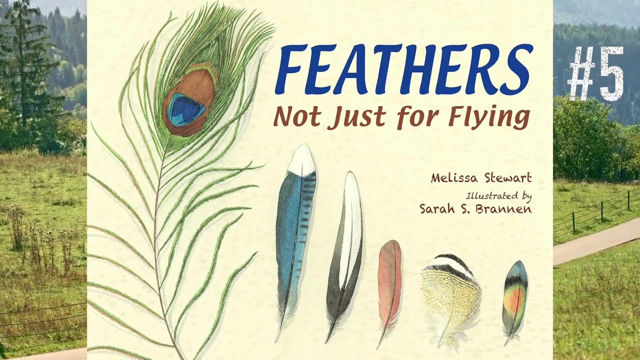 perspective, Young readers will learn all about worm habitats anatomy and their vital role in helping plants grow. Number five is Feathers, Not Just for Flying Feathers highlights 16 birds and the remarkable ways they use feathers beyond just flight, like warming, cooling, protection and 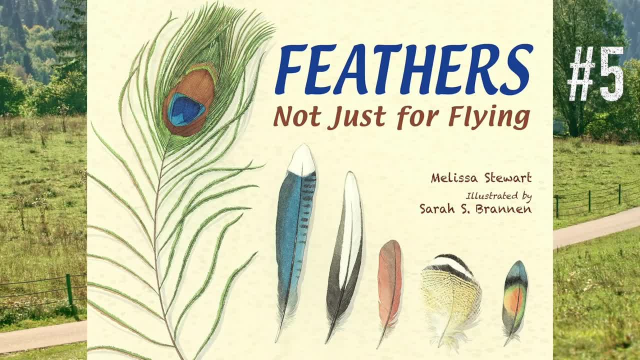 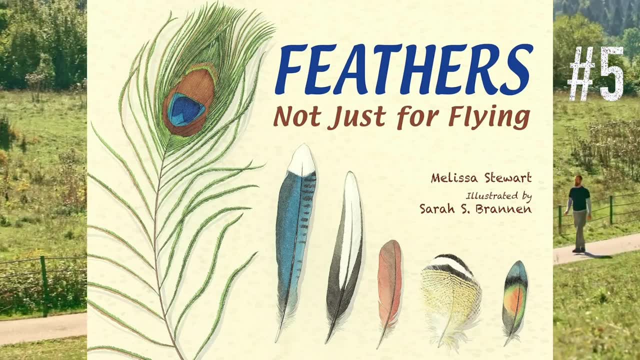 more Watercolor illustrations showcase life-size feathers. compared to everyday objects. Feathers is an elegant introduction to feather functionality that will fascinate kids with its insights into birds. Number six is The Kids Guide to Birds of Minnesota. This book introduces kids to the birds. 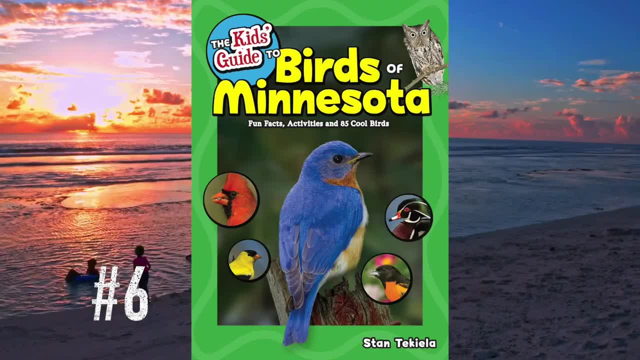 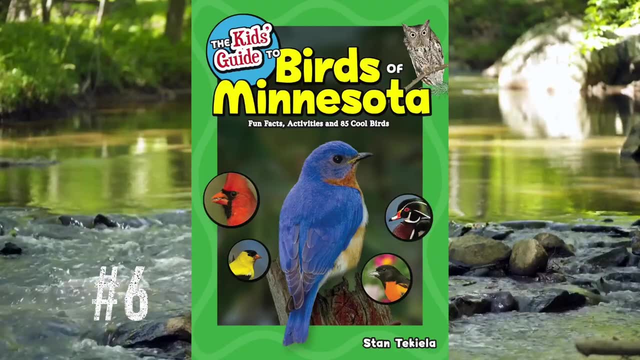 of Minnesota: fun facts, activities and 85 cool birds Calling all young bird watchers. Stan Tequila's Kids Guide to Birds series is a must-have for budding birders, With colorful photographs and fun facts about the most common birds in your state. 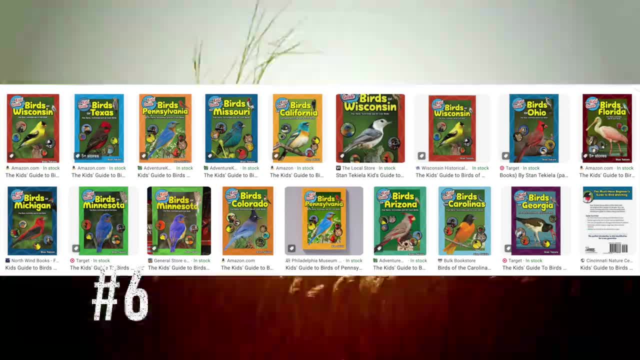 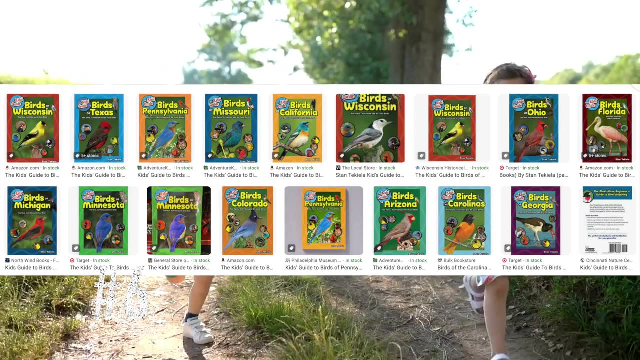 these books make bird watching easy and engaging for kids. Kids will love the cool tips on attracting local birds and hands-on activities like building birdhouses. Tequila's passion for birds is a real joy to read And, even if the book is a little bit contagious, his kid-friendly field. 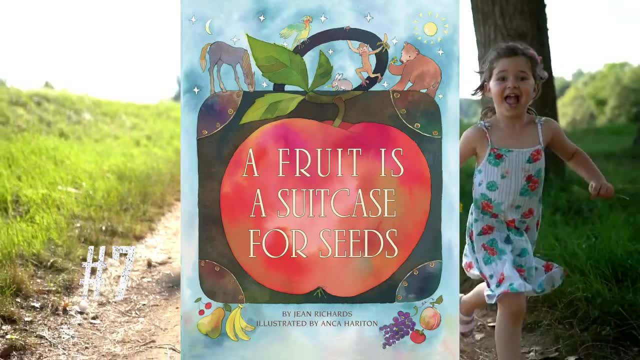 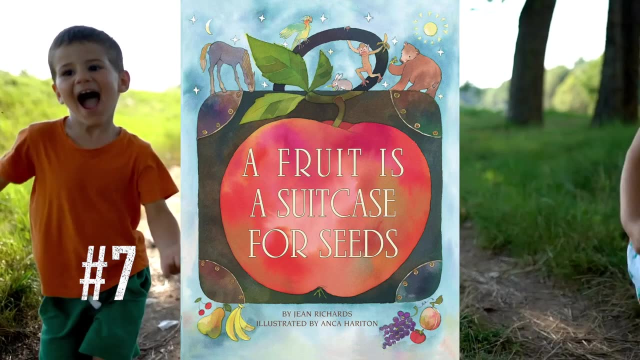 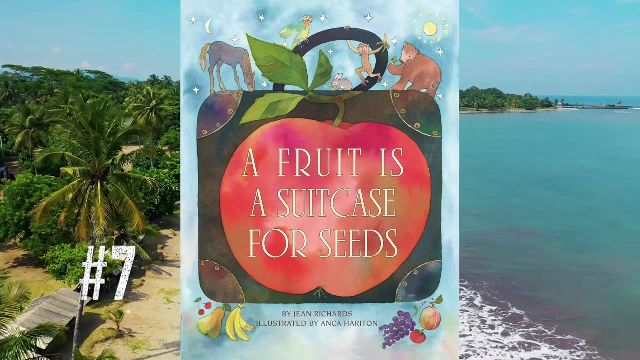 guides will turn kids into expert birders in no time. Number seven is A Fruit is a Suitcase for Seeds. A Fruit is a Suitcase for Seeds uses delightful prose and watercolor illustrations to explain seed anatomy and dispersal in a kid-friendly way. This book follows the journey of seeds packed. 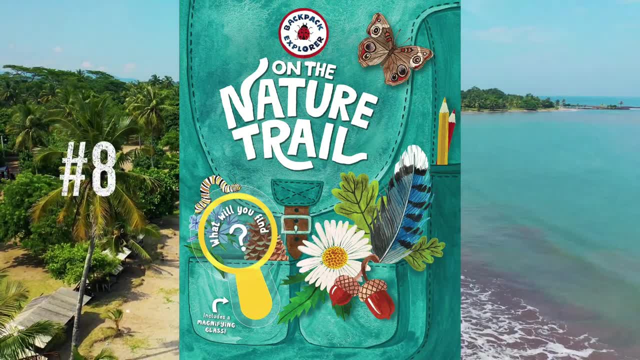 in their suitcases fruits as they spread to new places. Number eight is Backpack Explorer On the Nature Trail. What good is backpacking if you're not a backpacker? This book is all about backpacking, and I'll be right back. 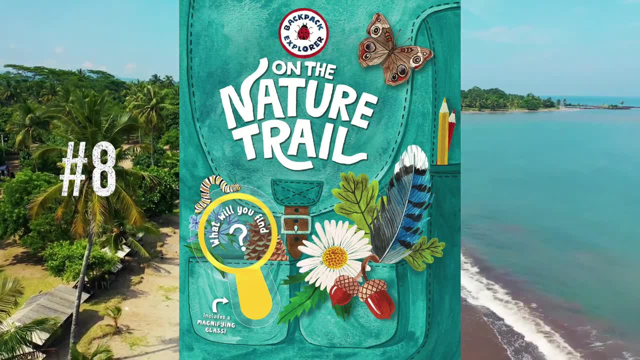 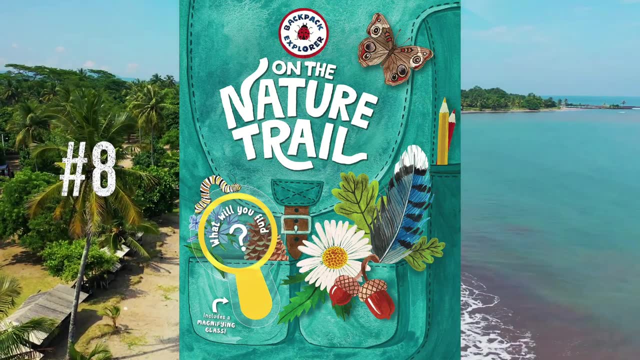 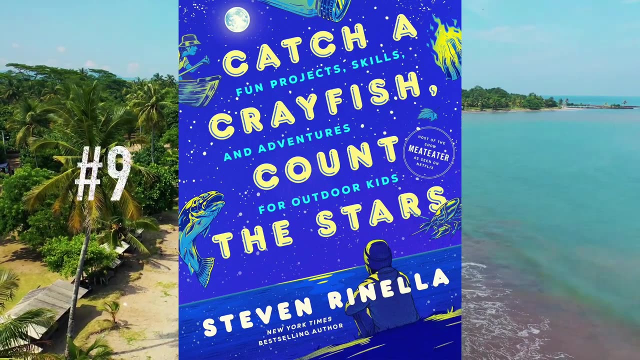 will you find. This interactive field guide encourages hands-on outdoor exploration wherever you are. Seek and find lists, art projects and discovery games. engage young learners to look closely at birds, bugs, plants and more. Number nine is: catch a crayfish, count the stars. 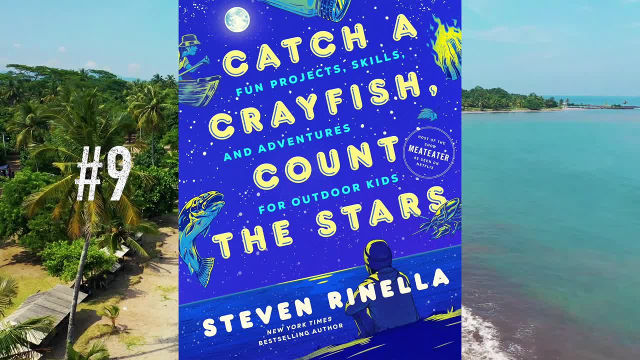 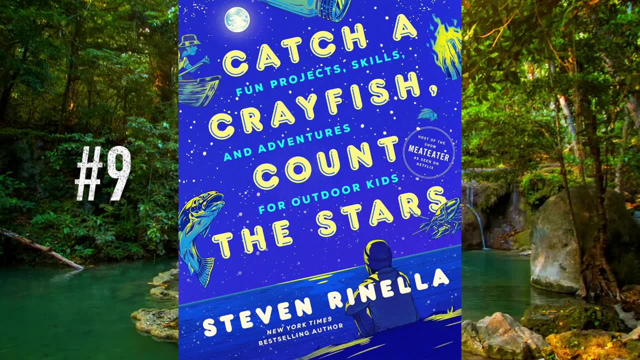 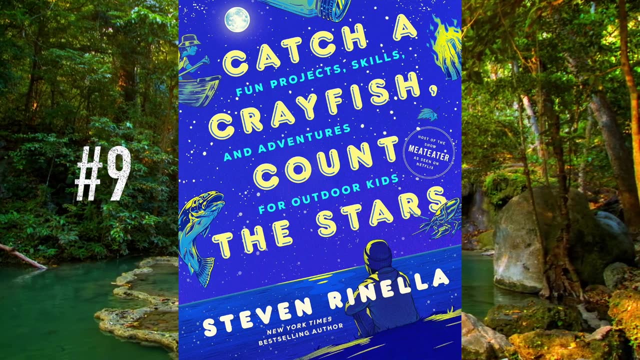 fun projects, skills and adventures for outdoor kids. Packed with fun hands-on outdoor activities like tracking animals, fishing, stargazing and more, this book will inspire kids to explore the natural world around them. Rinella makes learning active and engaging, imparting real skills while 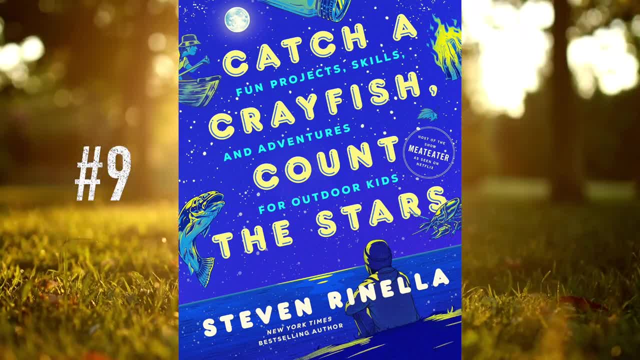 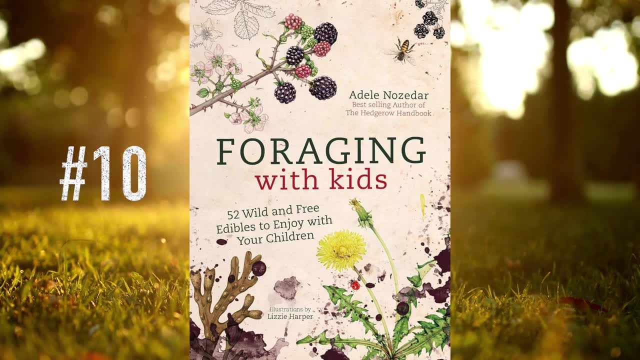 sparking wonder. It's the ideal guide for young adventurers ready to get outside and get their hands dirty. Number 10 is foraging with kids: 52 wild and free edibles to enjoy with your children. This book teaches kids how to identify and use 52 common edible wild. 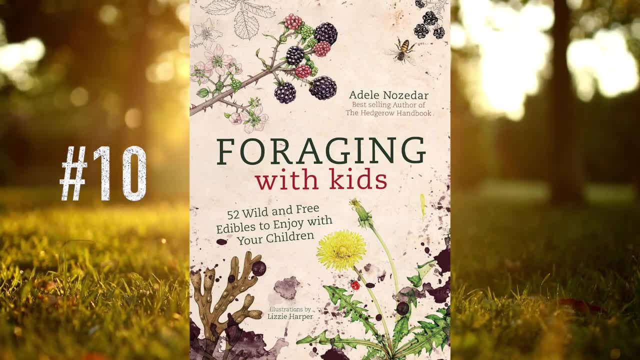 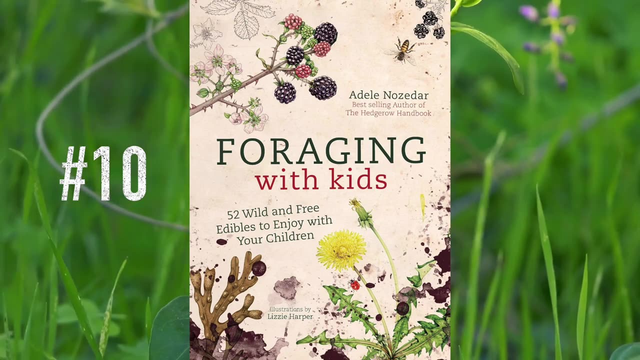 plants to create a healthy and healthy life, With creative recipes and projects to make from their finds. Foraging encourages hands-on learning, outdoor exploration and an appreciation of nature. With kid-friendly tips and beautiful illustrations, this book makes foraging a perfect family activity. Number 11 is Katia's book of 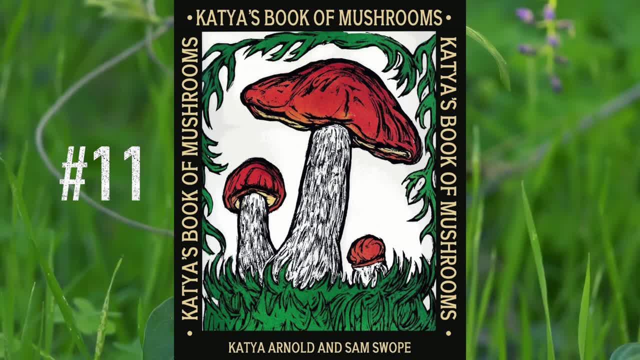 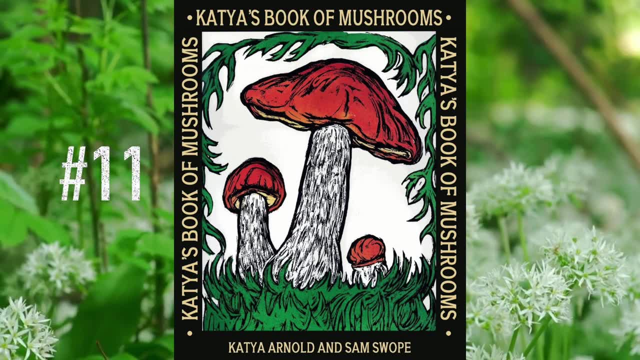 mushrooms. With hundreds of mushroom varieties, beautiful illustrations, fascinating facts and family foraging stories, this book makes mushroom hunting feel like a treasure hunt. Number 10 is foraging with kids: 52 wild and free edibles to enjoy with your children. 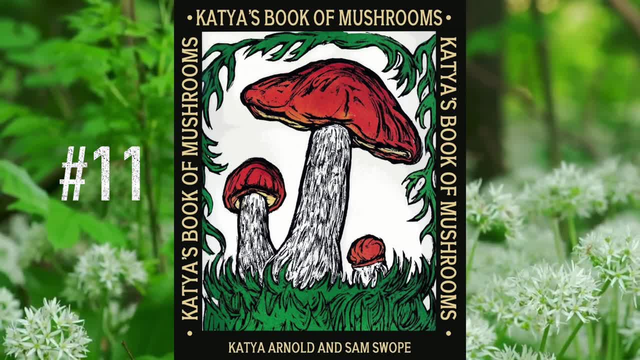 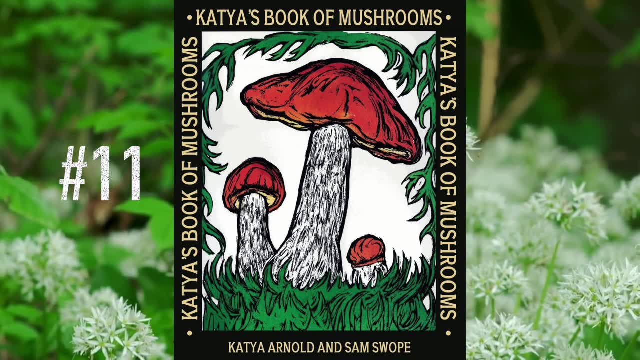 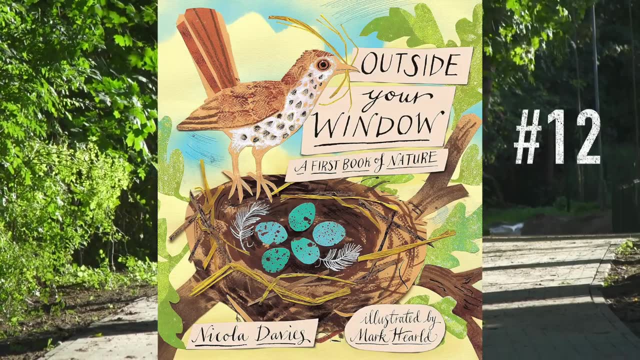 Kids will learn how to identify edible mushrooms, as well as appreciate the beauty and science of fungi. Katia Arnold's infectious enthusiasm and passion jump off the page, sure to inspire the next generation of mushroom lovers. Number 12 is Outside Your Window. a first book of nature. 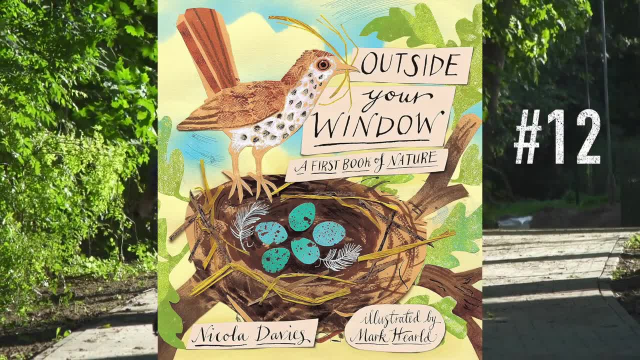 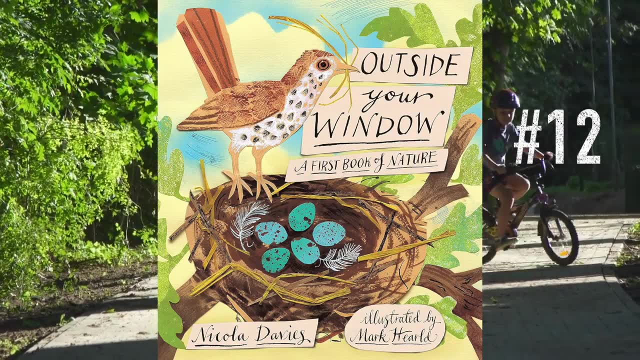 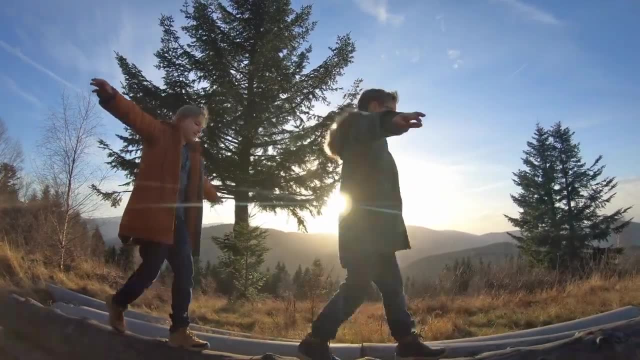 This gorgeously illustrated poetry book captures a child's joyful interaction with nature's beauty, from buzzing bees to snowy bird tracks. This book is a beautiful stepping stone to connect kids to the nature around them. There you have it: 12 incredible nature books that will inspire your love for the outdoors and ignite your curiosity. 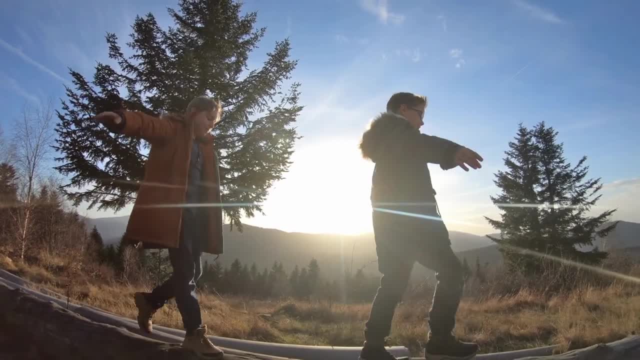 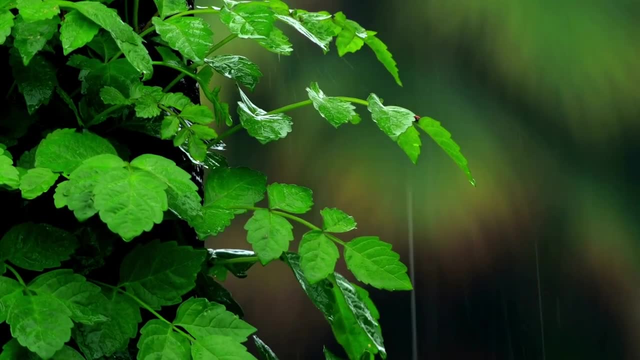 about the natural world. Whether you're foraging, birdwatching or simply exploring your backyard, these books are your companions on a journey of wonder and discovery. Happy reading. If you enjoyed this video, don't forget to like and subscribe. See you in the next video.